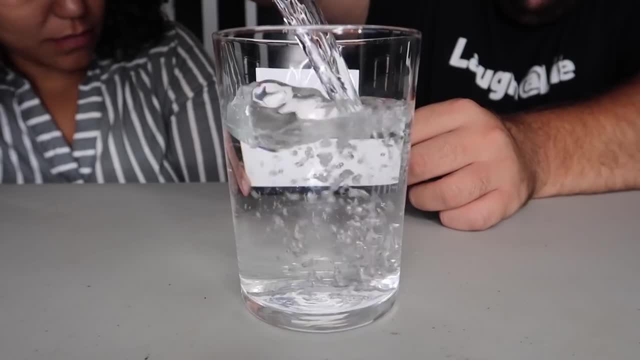 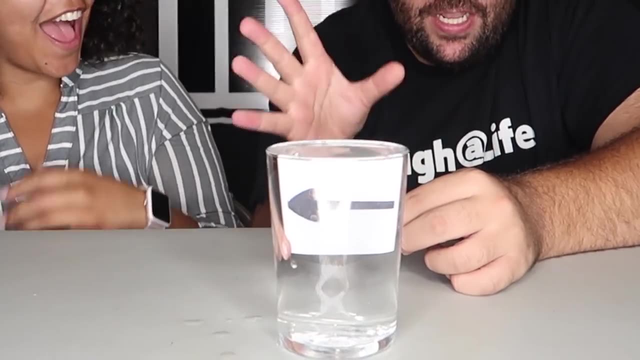 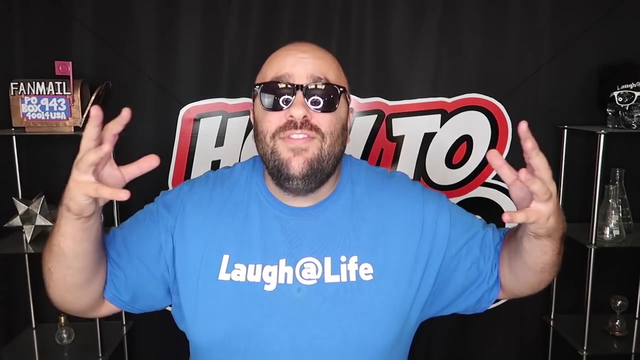 what happens. What's the arrow for Whoa? How did that even happen? Just like that, the arrow changes direction. Are you seeing this Whoa that looks so crazy. Alright, here's how it's done. I'm about to reveal the secret. 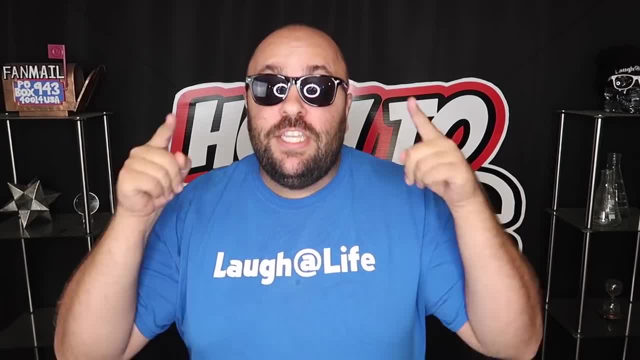 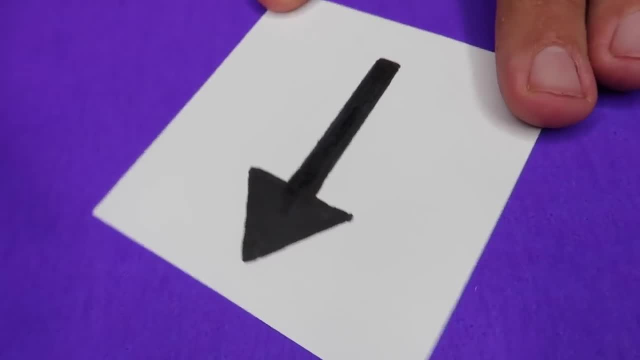 The secret to this trick is extremely simple, and I'll teach you how it's done right now. The first step in setting this up is to draw a arrow on a piece of paper just like this, And the rest is pretty self-explanatory. You take a glass. you want to make sure it has rounded edges. 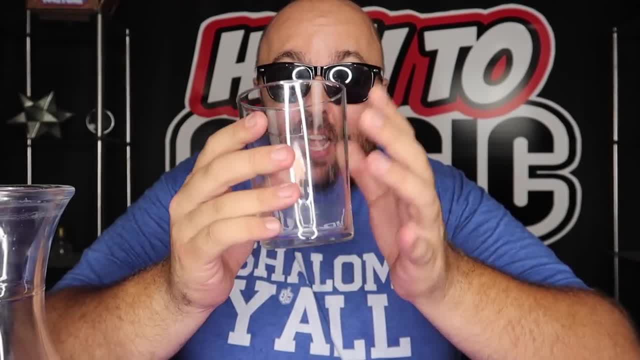 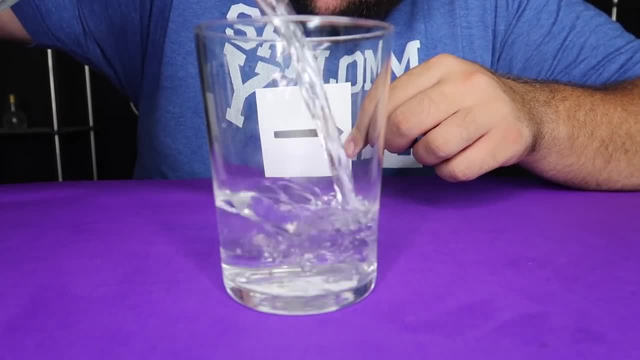 not like a square glass or anything like that, because the rounded edge is actually what's going to create the illusion of the arrow reversing direction. So think about the glass of water like a magnifying glass and when you hold the piece of paper at the right distance. 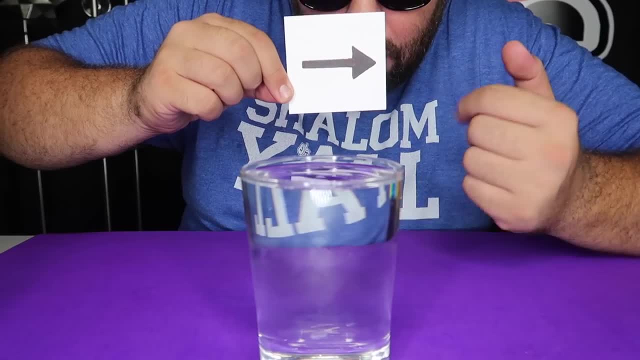 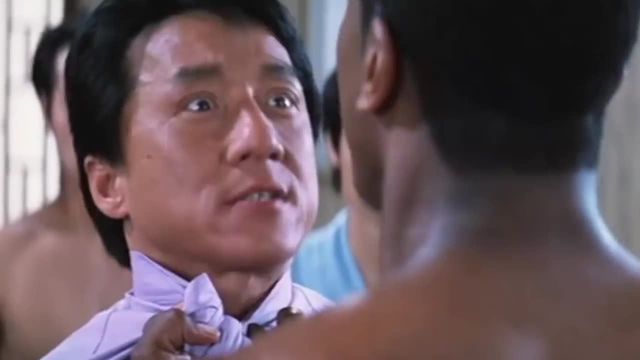 behind the glass it almost creates a lens effect. Up here it's pointing this way and as soon as it goes behind the glass, the arrow reverses directions and points that way. I go that way, you go this way, Yes, Okay. 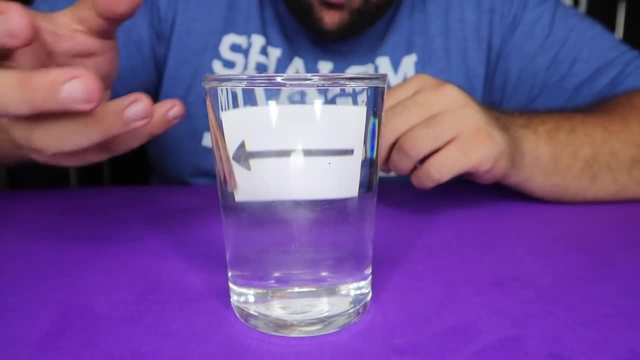 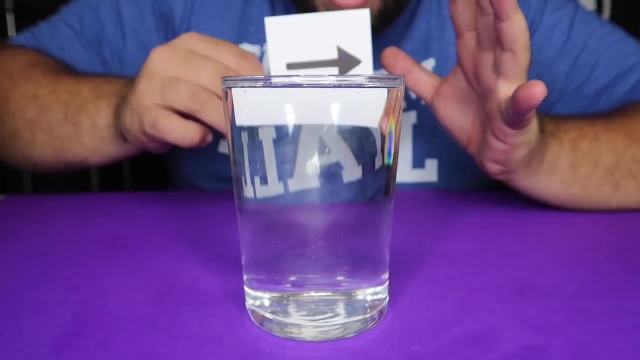 This is because the light coming into the glass reverses directions when it comes into the glass and when it exits it, giving us what appears to be a reverse image of the arrow. So fill up a glass with water, grab a piece of paper and try this out at home. 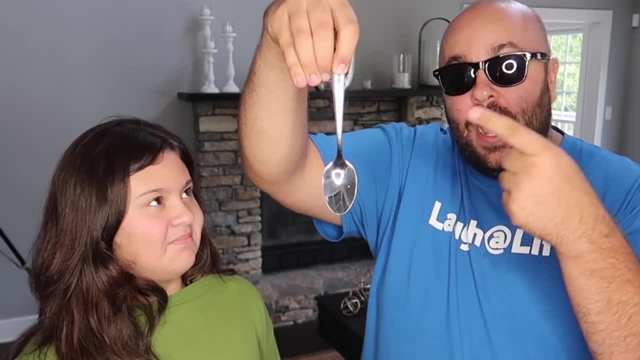 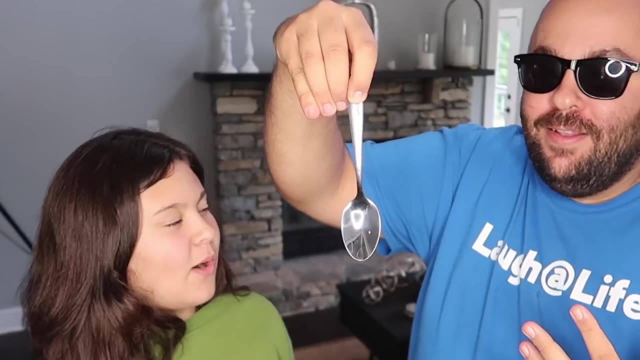 Okay, Ava, this is my sad spoon. He actually cries. My spoon cries. Why is he sad? Well, he's not sad, yet We have to make him sad. Why? That's bullying? It's just part of the trick, So check it out. 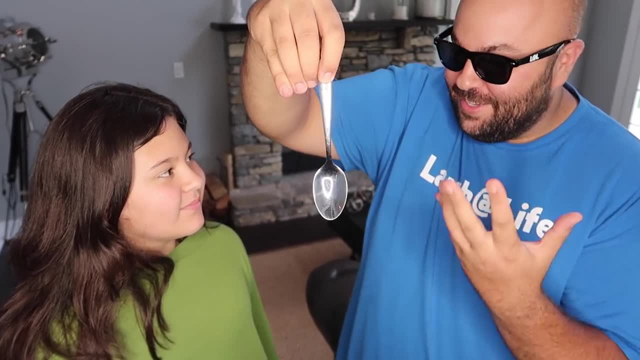 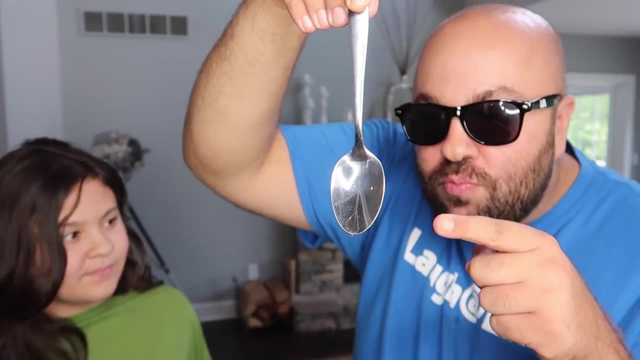 We have to be mean to the spoon in order for it to get sad and cry. So we say things to it like forks are better. People only use you to eat soup. I hope you get rusty. See, he starts to cry. Sad spoon. 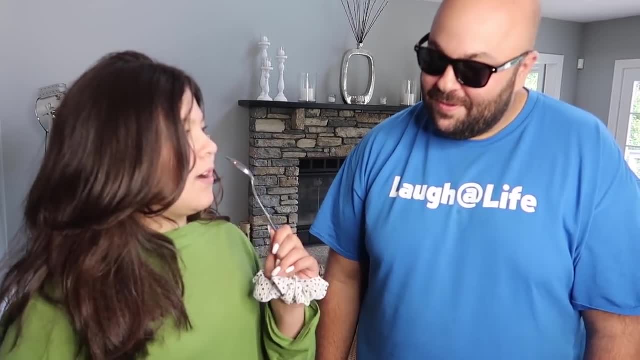 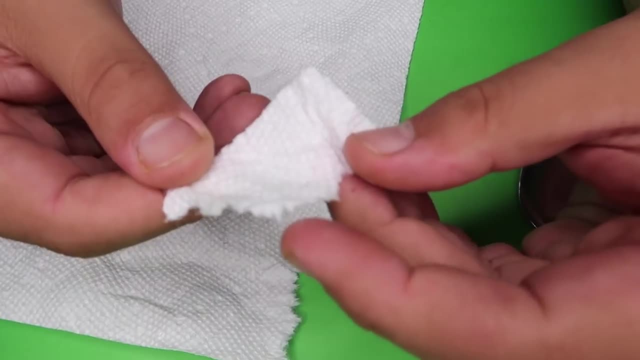 Here you can try it out. This spoon has powers. This is a super easy one that you can do at home. All you need is a paper towel and a spoon. Any spoon will do, And you're just going to tear off a little piece of paper towel. 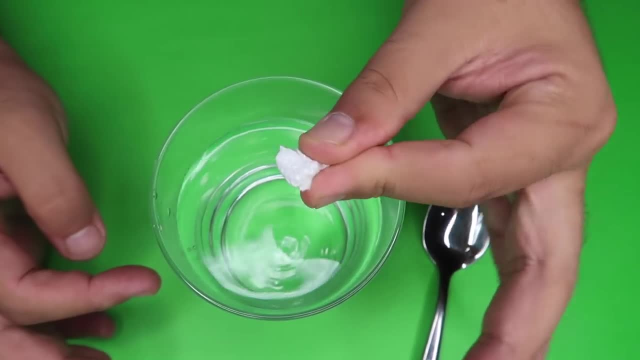 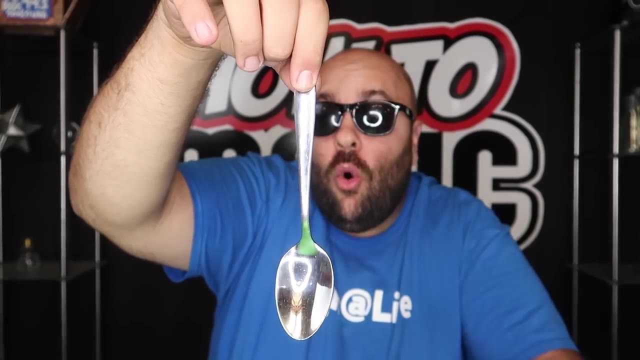 Before the trick starts, ball it up like this: Now, take that piece of paper towel and dunk it in water. This is what's going to simulate our spoon's tears. Now, when you hold the spoon, you're going to conceal the wet piece of paper towel right here behind the spoon. 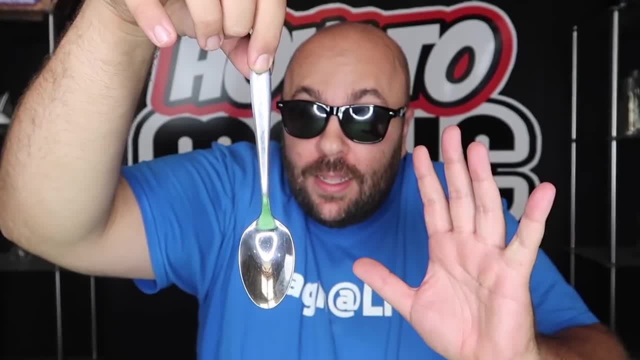 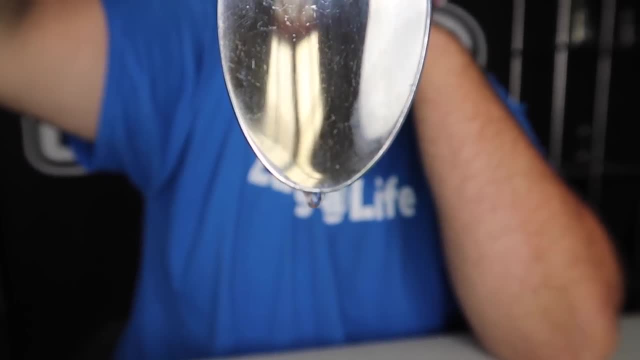 with your thumb, pressing it against the back, And you can hold it like this. Then, when you're ready to make the spoon start crying, all you have to do is squeeze a little and the water will drip down the back of the spoon and begin dripping right off the end, right here. 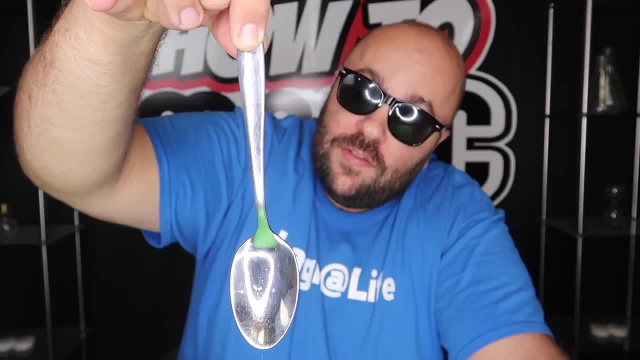 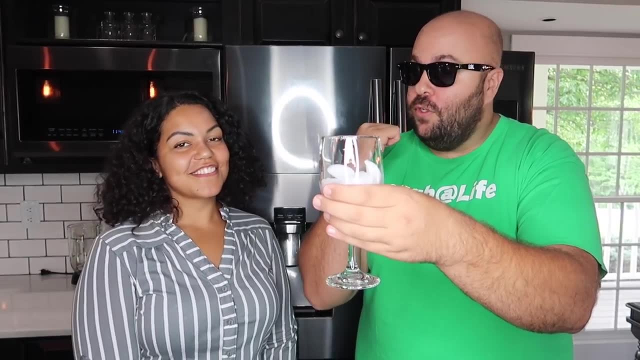 And it really creates the effect of the spoon just crying So sad. Try this one out at home. It's good for a laugh and it's an amazing trick. I've got a glass here. Did you actually know that the fridge makes wine now? 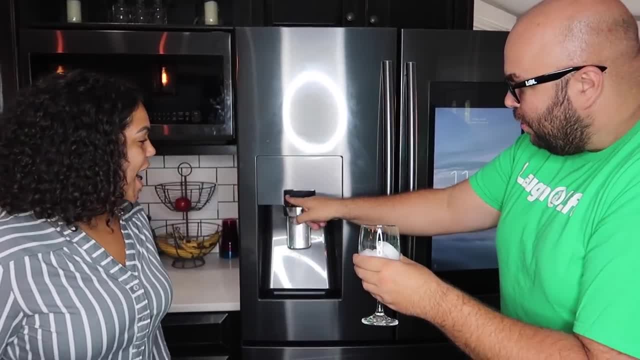 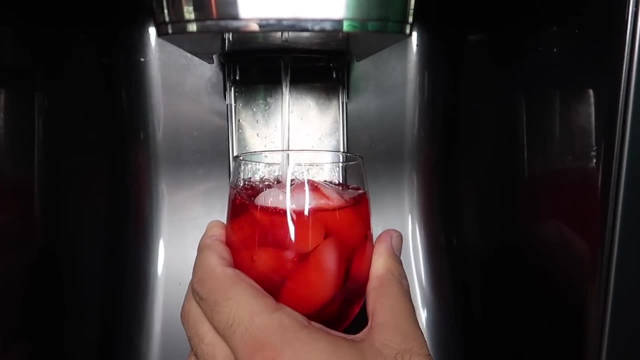 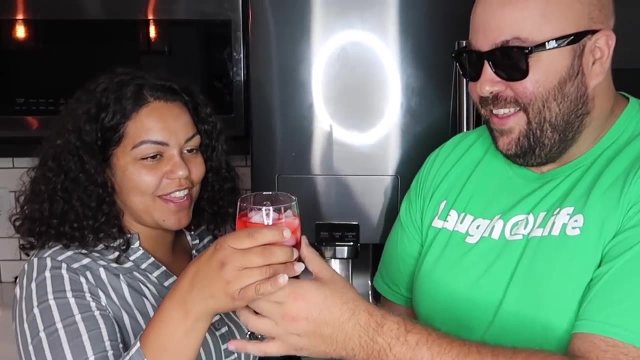 What? Yeah, check this out. If you just select water, Why, Watch? You're just not telling me this. That is not wine. You're joking. Where do you get this type of fridge? All you need to do this is a cup and some food coloring. 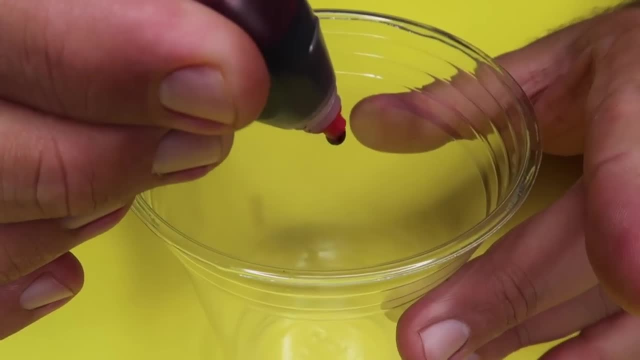 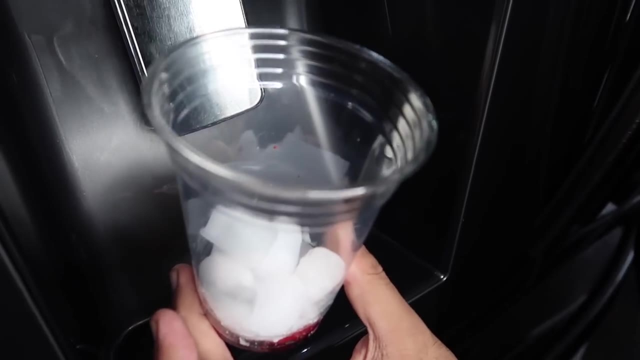 Before you present the trick to the audience, you're going to secretly put a couple drops of food coloring in the bottom of the cup. Next step: put some ice on top. The ice is going to help hide the food color in the bottom of the cup, and we're going to 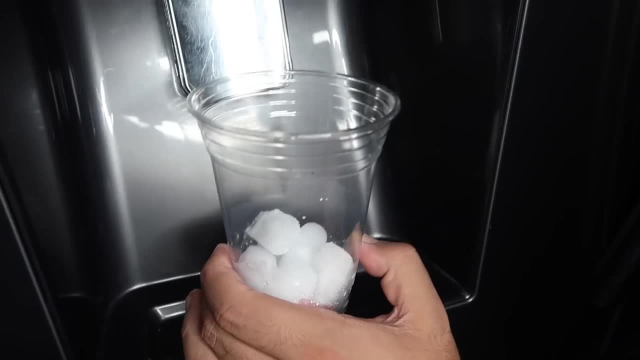 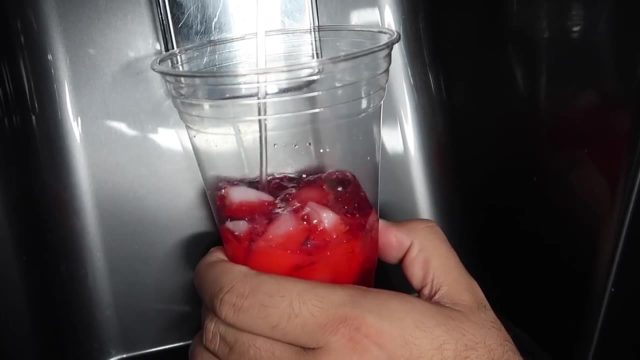 cover the very bottom of it with our fingers, just like that. Now your trick is set up and ready to go. you can present it to your audience. So hey, check this out. If I put some water in the cup, you can see it turns from water into wine. 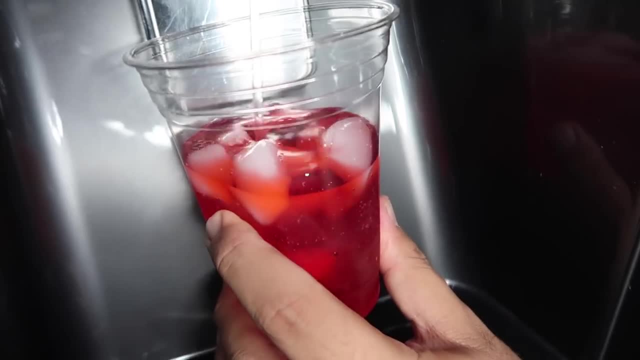 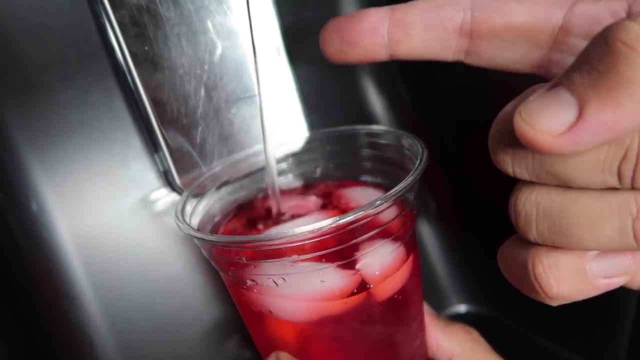 And as the water hits the food coloring in the cup, it's going to mix and really create this convincing illusion that it is just turning from water into wine. You get this nice visual of the stream of clear water and then it turns into red liquid. 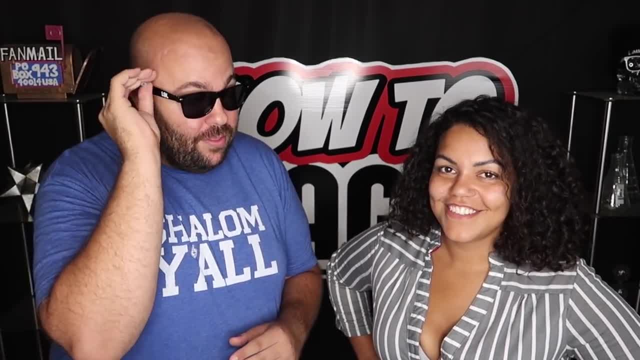 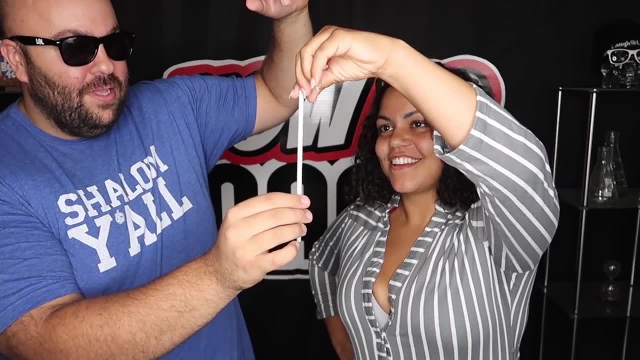 inside the cup. Okay, V, I have a cool trick to show you with. Do you This straw With a straw, If you will just pinch it right here at the top, just like that. Hold it like that, All right. 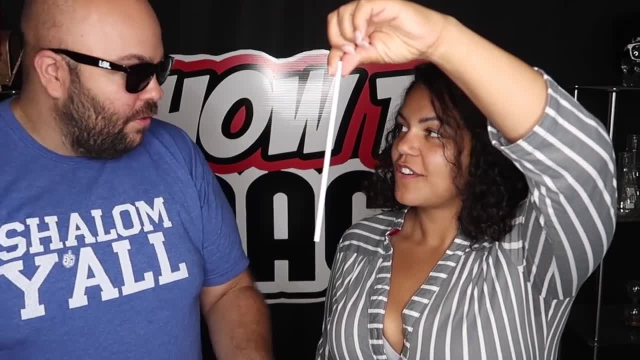 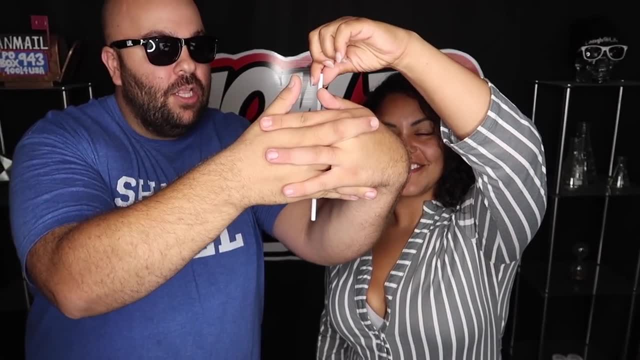 Now, if you were to just let go of it right now, it would definitely just fall to the ground right, Because of gravity. Yeah, All right, But look, if I take my hands like this and I hold it in front, just let go of the straw. 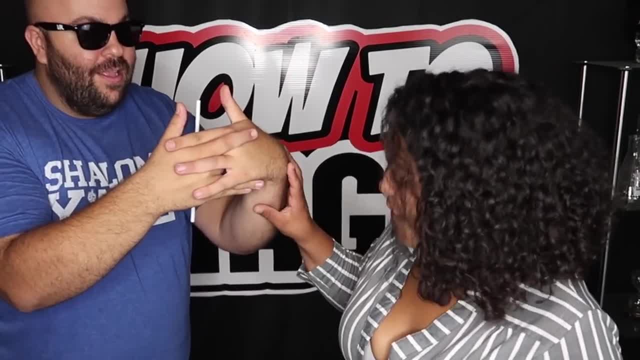 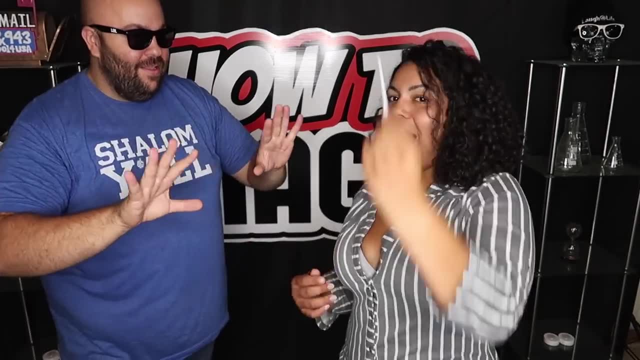 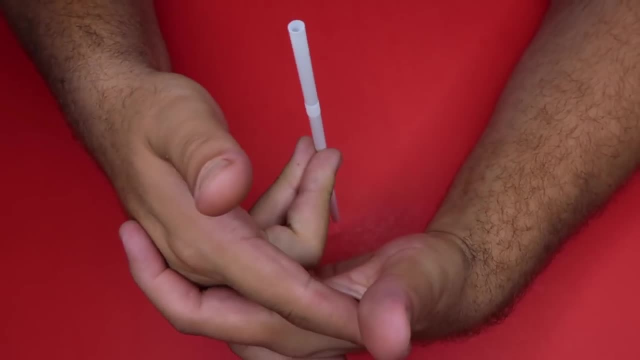 just like that. Look It floats. Oh what In mid-air. Just like that, What, What, What. Show me how, I'll show you. and you right now. Okay, here is the secret to the magic floating straw trick. 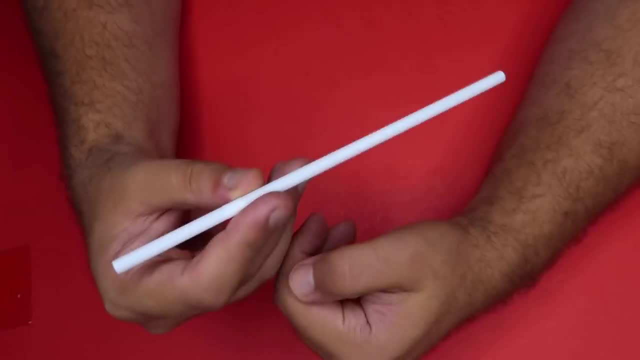 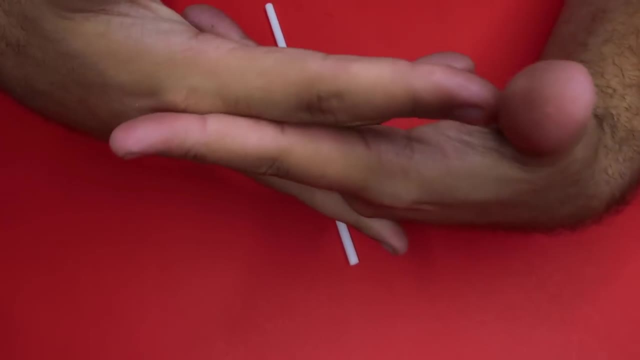 This is totally impromptu. You can set this up anytime, anywhere, and you don't have to use a straw. You can use a pencil or a pen- any object that you can trap in between your fingers. You're going to interlace your fingers like this, leaving these two middle fingers on. 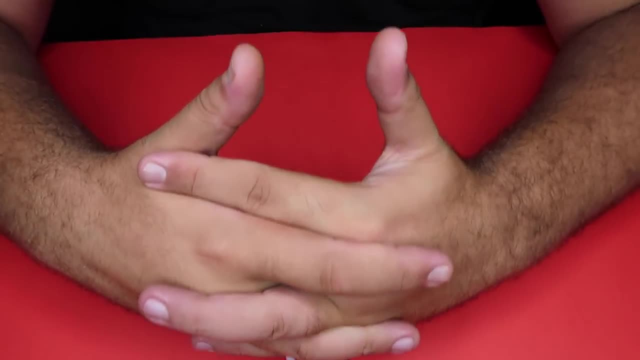 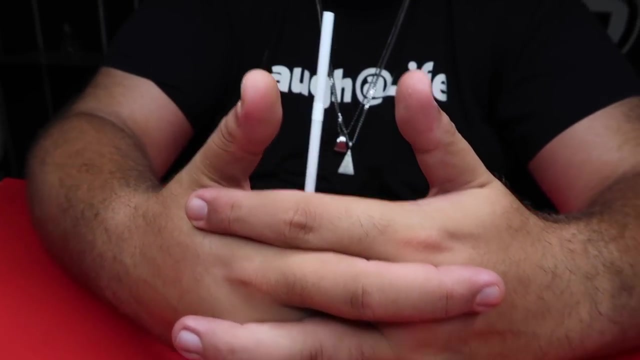 the hands protruding. That way your hands look normal from the front, but you have these two fingers free to manipulate. So just practice the movement until it looks nice and smooth and it looks like the straw is just floating behind your hands and you want your front interlaced fingers to remain. 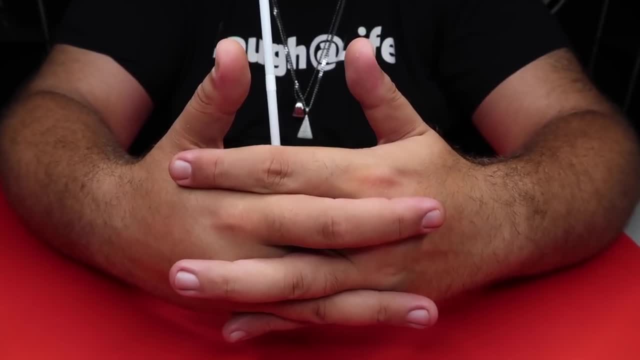 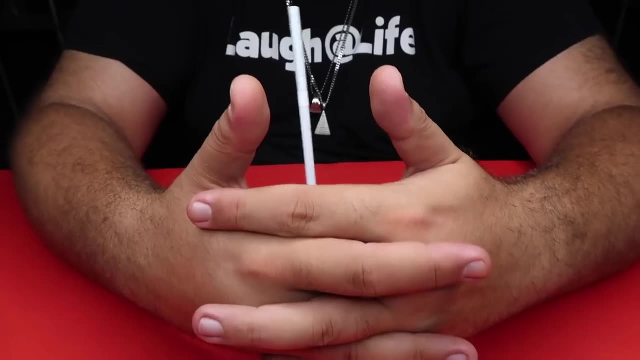 as still as possible. so it looks like the straw is just moving and your hands are staying still. There's no way that you could be manipulating it with your hands, and it really looks like the straw is just floating in mid-air. This is the magic coin box. 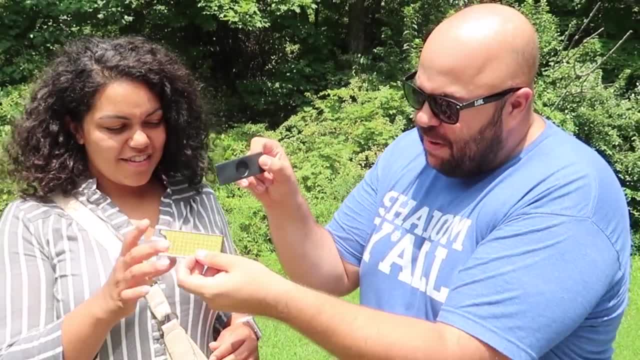 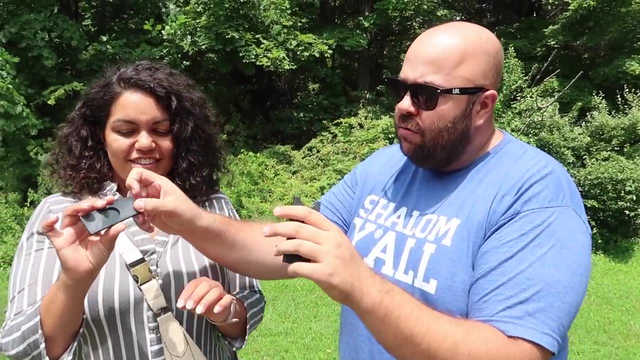 Check this thing out, Vy. It's just a little plastic box. Yeah, You can inspect it, It's legit, There's nothing tricky. Yeah, it's cool. right, Check it out. Nothing in my hands, So check this out. 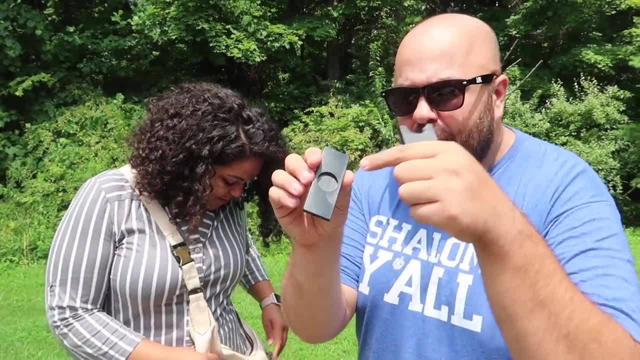 Do you have a coin on you Like a penny? Yeah, we're going to put like a penny or a dime or something like that, Anything. Yeah, a penny would be perfect. if you have a penny, Ah, perfect, All right. 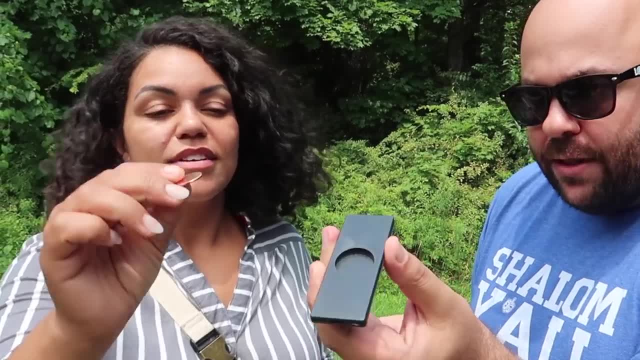 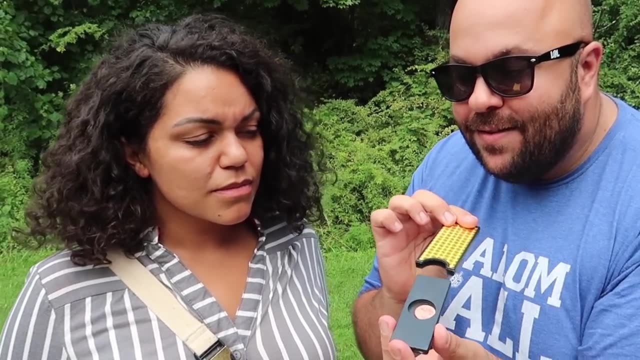 Go ahead and put it right inside our little coin tray there. Okay Boom, All right, You see it goes in. Now I'm going to take the little tray and I'm going to slide it inside this box. You can see there's nothing inside it. 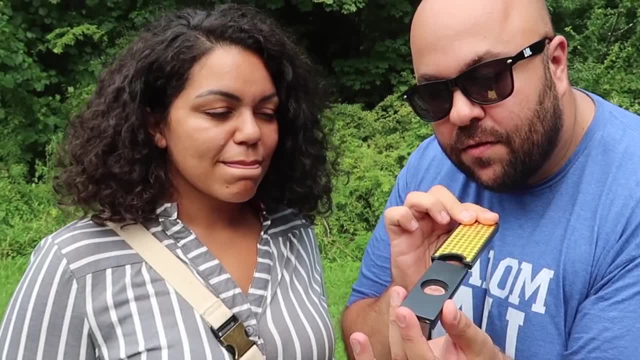 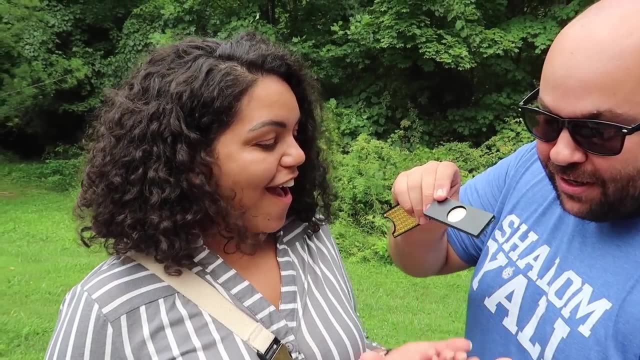 A little pocket. Yeah, I like that. All right, Watch, Slide it in, like this: One, two, three. Look It changed What Into a quarter here, Hold out your hand. Ah, yeah, What is that? 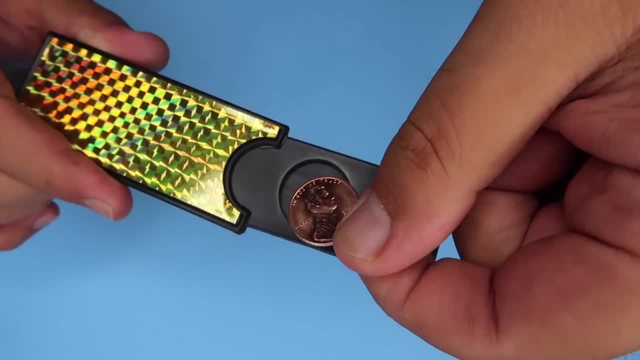 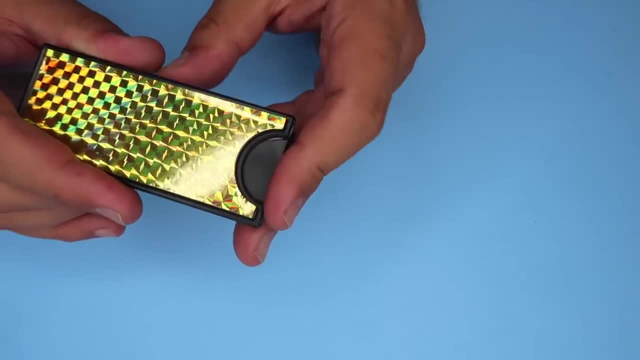 It's 25x your money. The secret to this one is very simple. This is our coin slide tray, available at evaneratvcom. You can take a coin, put it inside, slide it in like this and it will magically change. 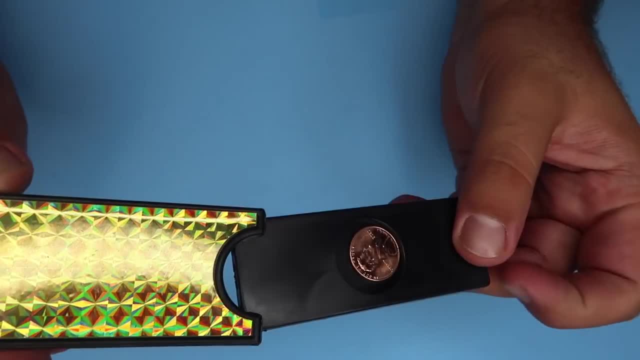 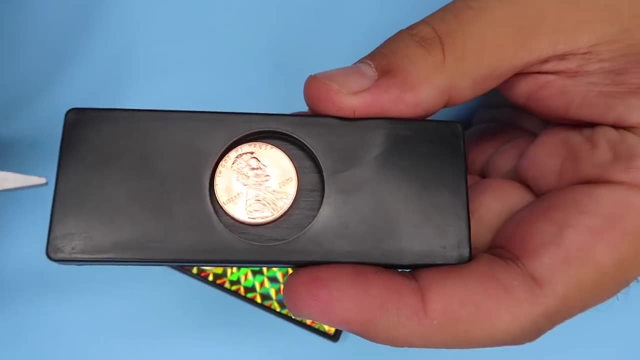 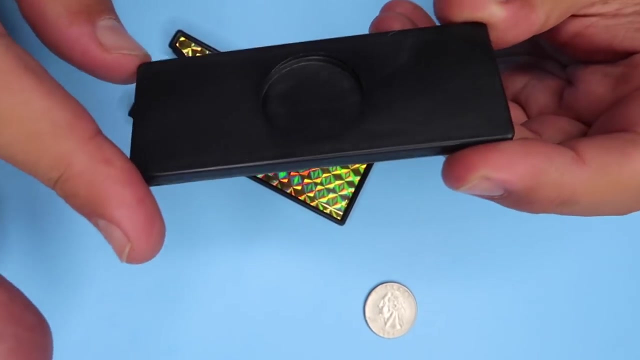 it into a different coin. Or, as you saw in the performance, you can use it to make a coin appear Or disappear, Just like that. Inside the tray is a hidden secret compartment, so you can have a coin here and as you slide it inside the little magic box, the tray will slide just like this and it appears as though. 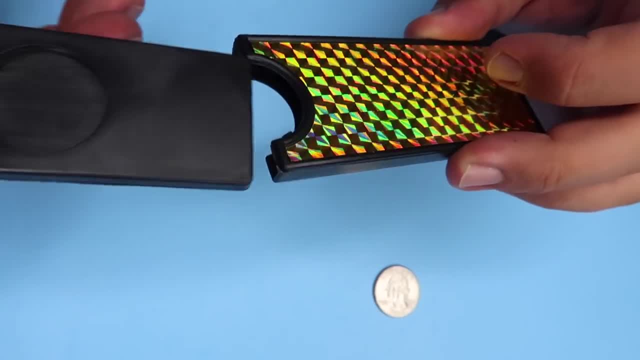 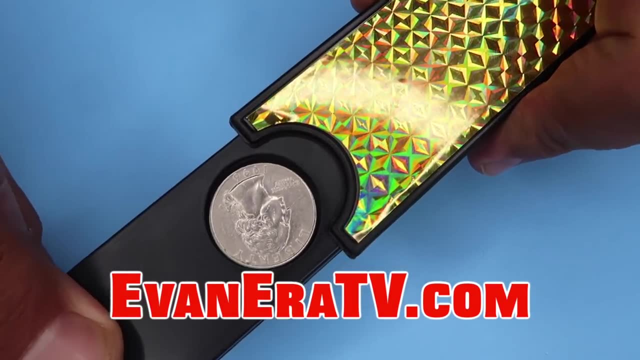 the coin has just magically vanished. You can then reverse that process to make the coin reappear. It's a super easy trick that anyone can do. Head over to evaneratvcom. They are available now, or stay tuned for the end of this video for a chance to win one. 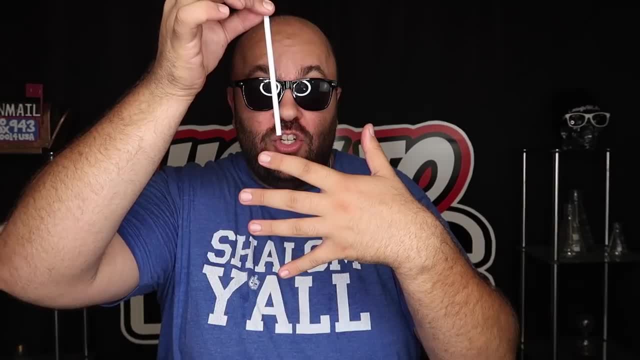 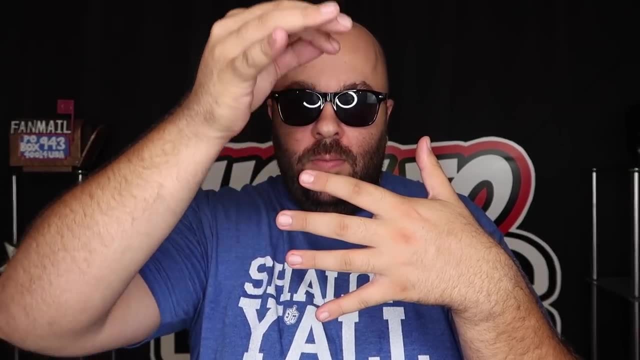 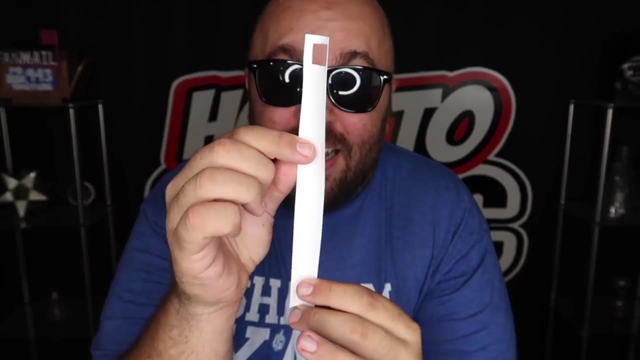 in this week's giveaway. All right, it is bonus. trick time: Watch the straw. Here's how it's done. This little piece of plastic: right here. I cut this out of a shower curtain rod cover. You're going to wedge this in between your hand and your face. 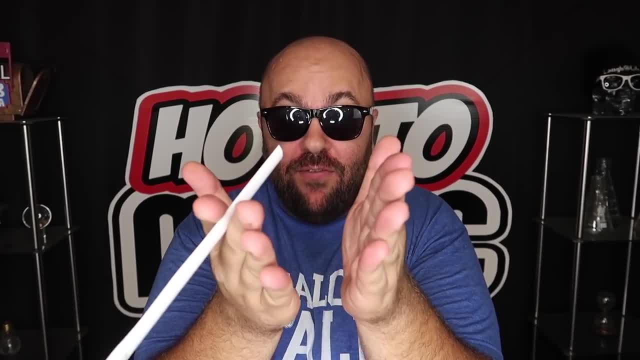 It's very angle sensitive. You have to make sure the person is watching it directly in front of you. It's a great thing to film on your phone or on a camera and send to someone. So here's what the audience is not seeing. 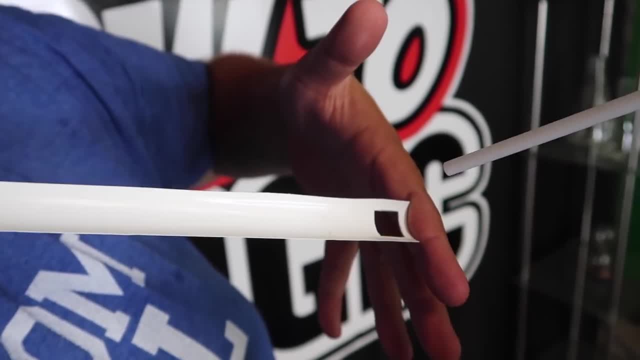 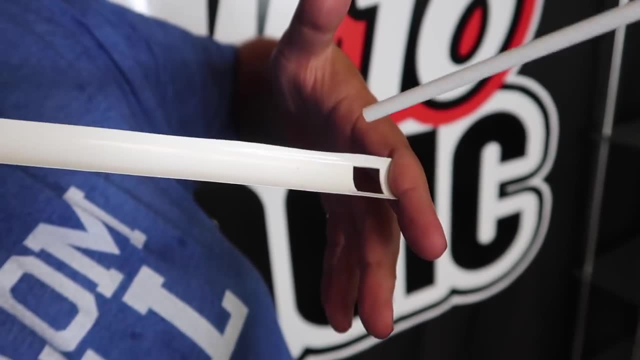 When the straw first slides behind my fingers, it's going right through that hole there- That is why you're able to see it through my fingers- and it just slides so easily up and down. Then, whenever I want to make it vanish, all I have to do is kind of lay it right on this. 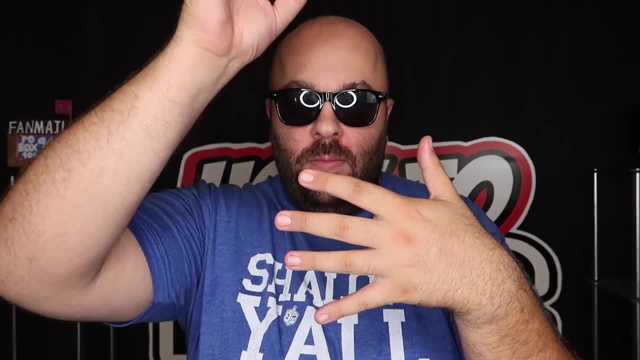 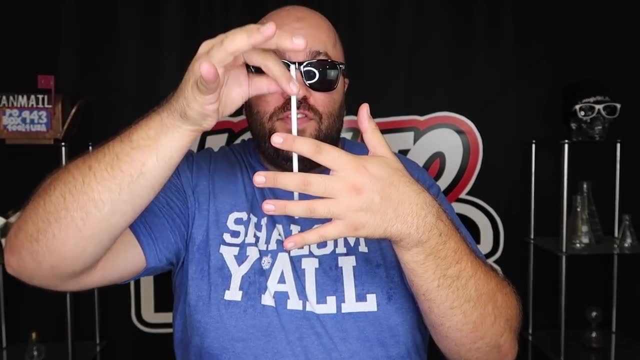 little tray. That is how I'm able to let go and it looks like the straw just vanishes behind my hand. Best to set this up and practice in a mirror until it looks smooth, so that you go from this visual of the straw just going right behind the fingers to it really creating a 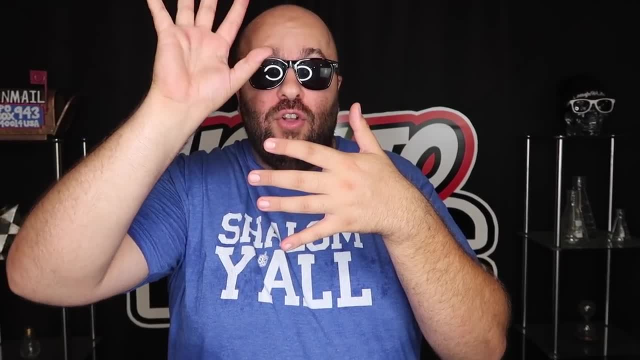 convincing illusion of the straw: The straw just vanishing as it slides behind your hand. All right, guys, that is it for this video. If you liked it, hit the thumbs up button and share it with someone who you think might like it too. 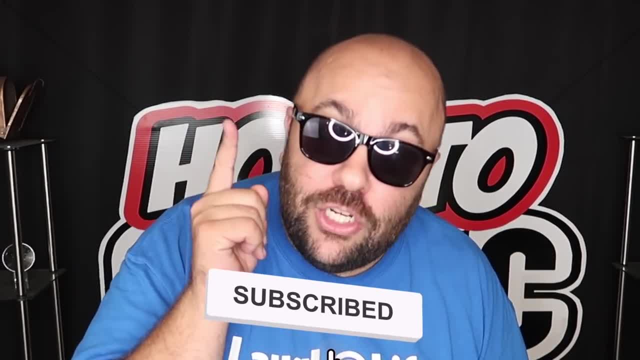 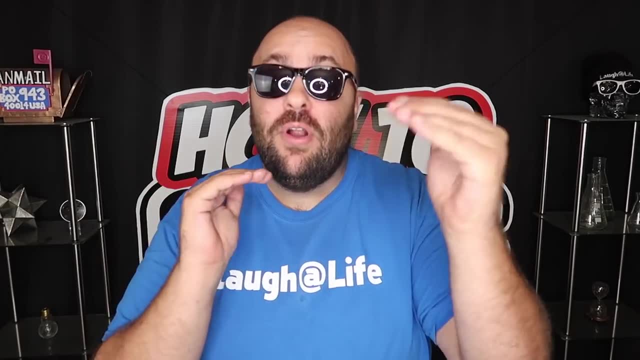 If you're new to our channel, be sure to hit that subscribe button and tap the notification bell so you see new magic videos like this every single week. If you want to go back and look at a specific trick in this video, it's been separated into. 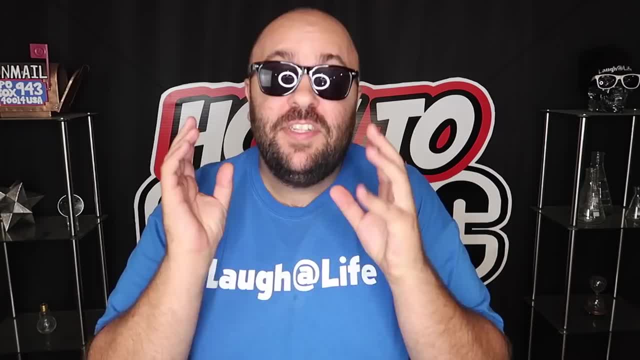 chapters so you can go back and get a refresher if you need to practice the steps. They're all laid out for you. And it is giveaway time. We do a new magic giveaway on every single episode of How To Magic, and this week is no.